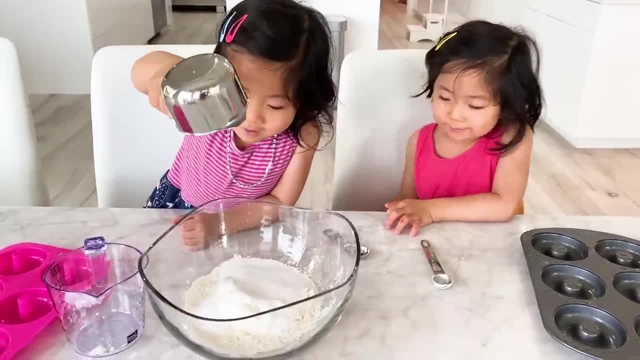 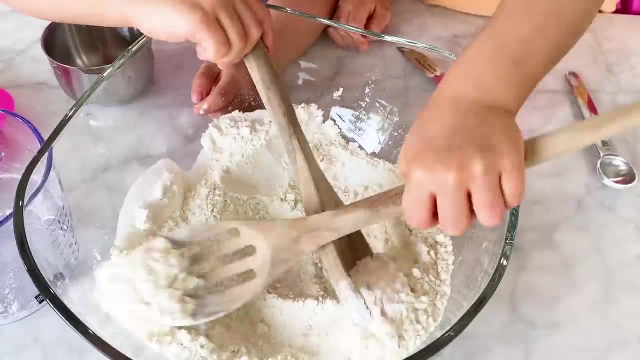 and now Emma's going to add the sugar. Woo-hoo, Yeah. so next is we've got to mix it together. Agitate, agitate, Good girls, There you go, Mix it together. Agitate, agitate, Agitate, agitate, Good girls, There you go, Mix it together. 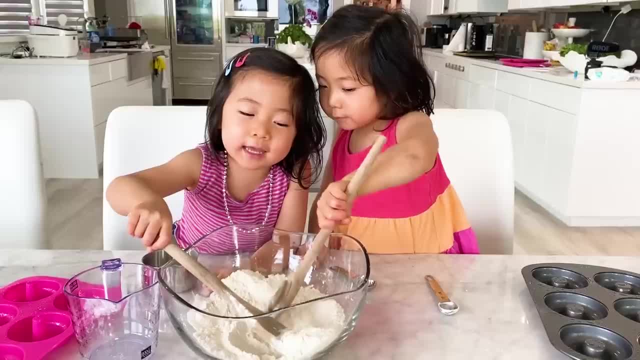 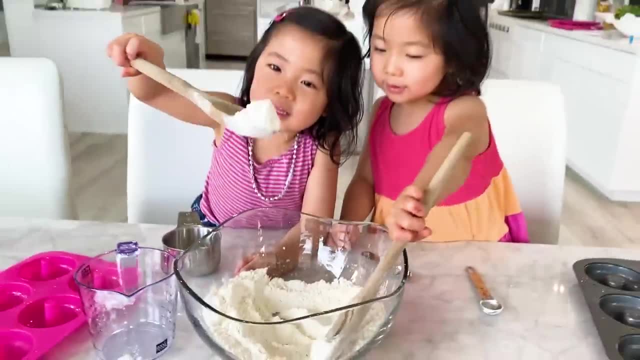 Agitate, agitate. Good girls, There you go, Mix it together. Agitate, agitate. That's right, Emma. Agitate means mix. This is your donut stick. Is it donut yet? No, Not yet. 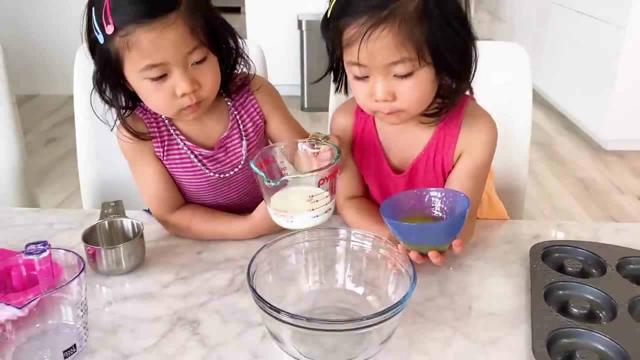 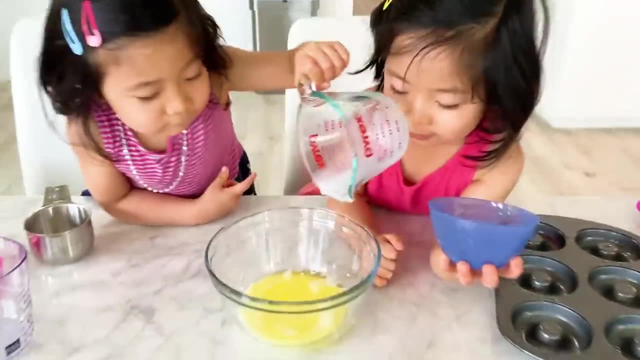 They've done mixing, so now for the next step. we get a different bowl. Emma's going to add the milk and Kate add the butter. Butter, Yeah, sure It smells so good. I love butter, Do you? Yeah? 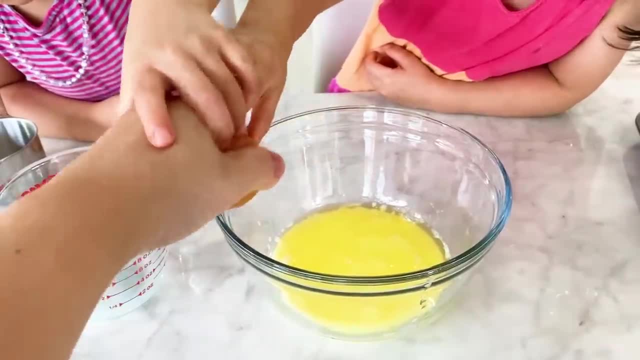 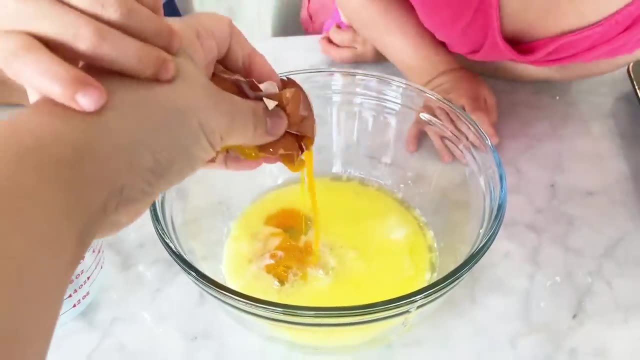 So I have an egg here. Mommy's going to crack the egg. One, two, three, Two, two, two, two, two, Crack. There we go, Mommy, that's how you do it. Yeah, Next step, mommy, have to put vanilla extract. Okay, you have to hold it out steady. 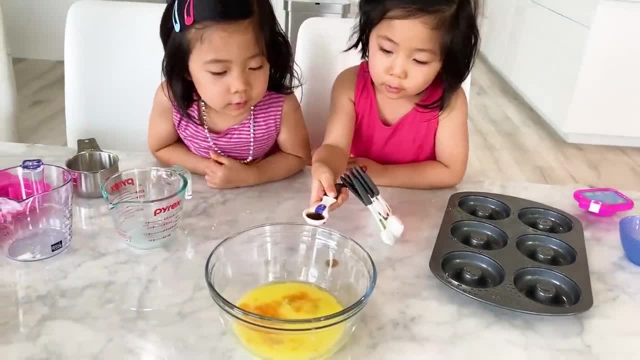 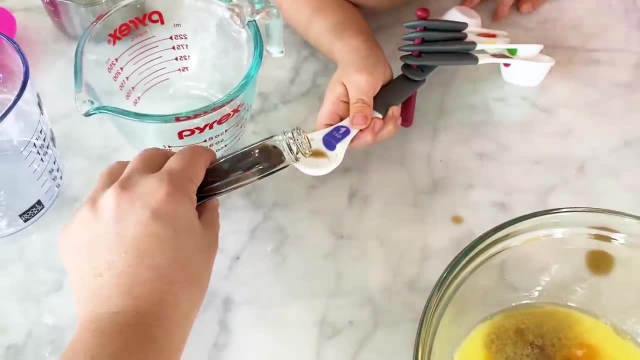 Okay, put it in. Does it need to drop? Yeah, Okay, Emma can do another one. Okay, There you go. This is liquid. It smells so good, Smells good. Okay, a little bit more for Emma. Okay, put it in. 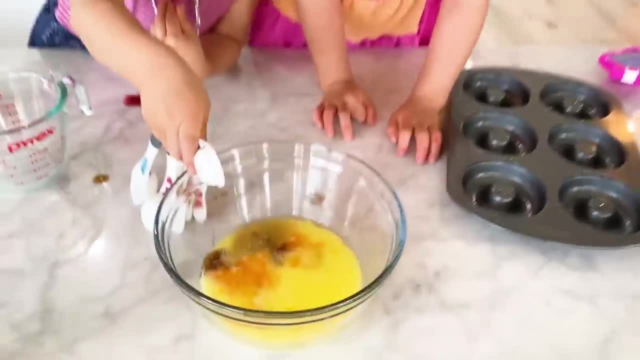 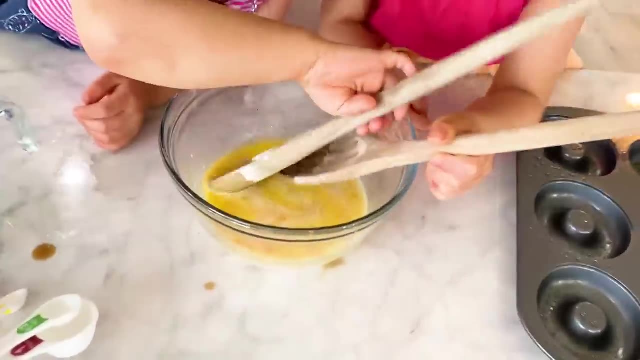 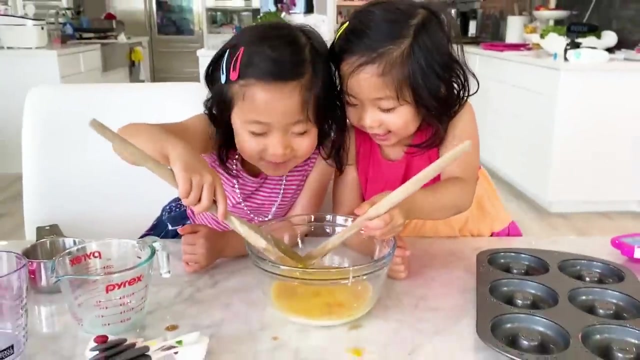 Okay. One, two, three, There you go. Wow, So now they're mixing it up. This is first. Try, maybe- Eh, it's not a soup. Try, maybe. Okay, now next, add that in there together. There you go. 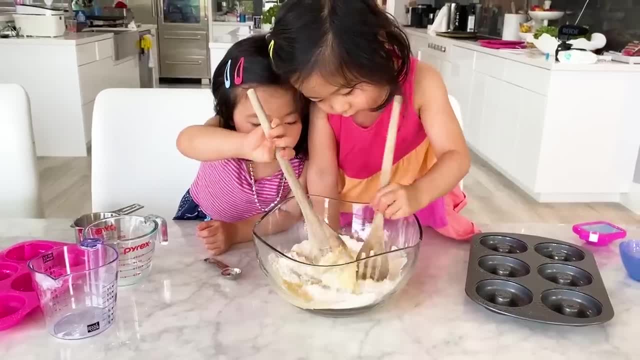 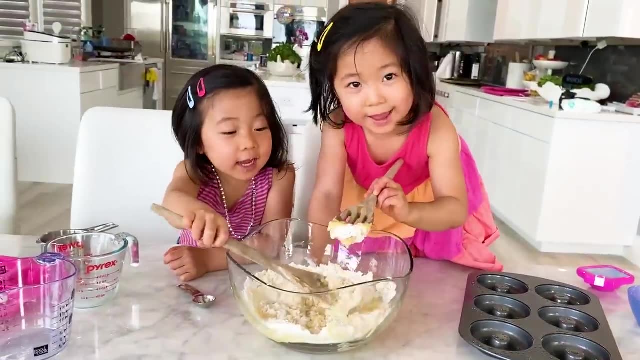 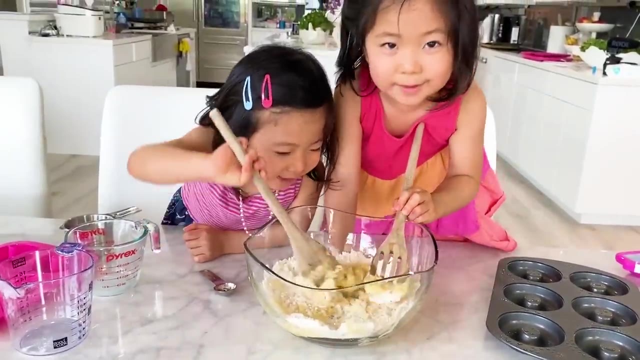 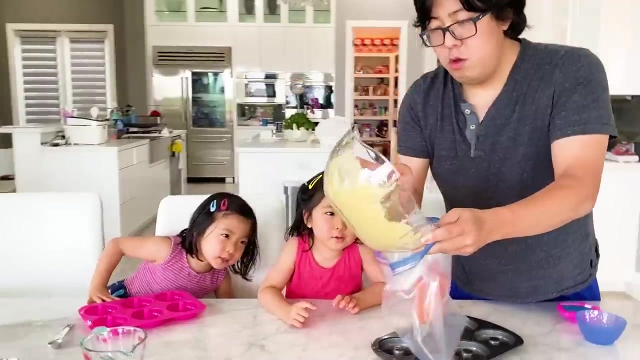 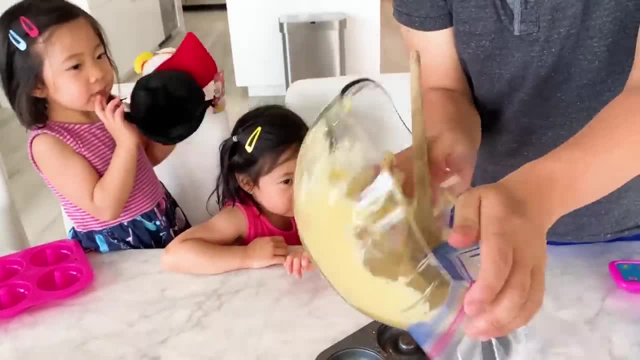 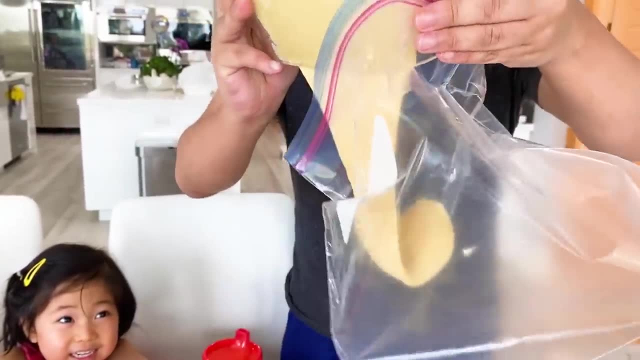 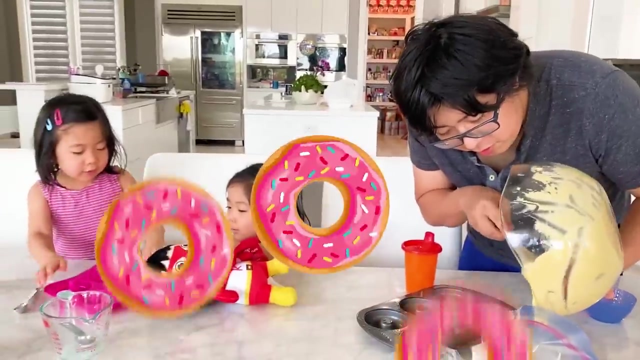 So next step, we have to put the donut mix into the Ziploc bag. Can you do it? There you go. Is it working? Yeah, Yay, It's working. Wow, What are you guys making? Donuts. 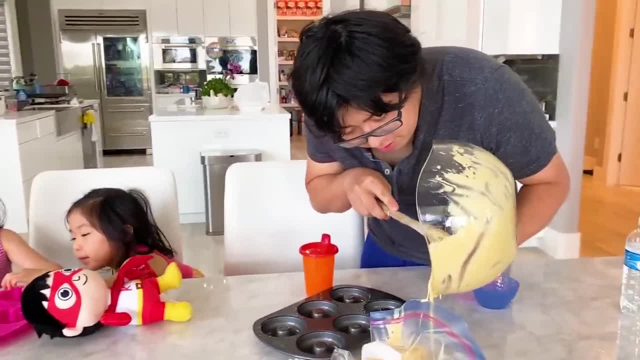 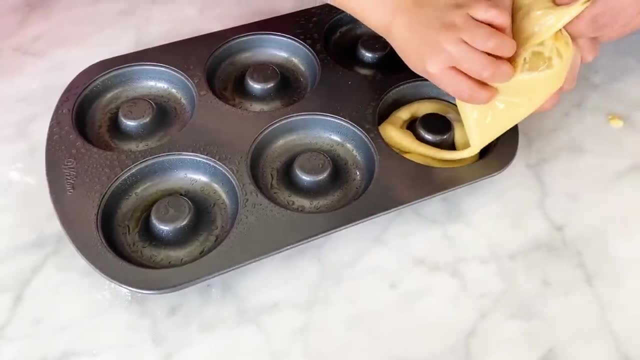 Donuts, What You want to try it later. Yes, So now we're going to squeeze into the mix. What are we doing? What are we doing? Maybe one more circle? Good, Okay, thank you. There you go. 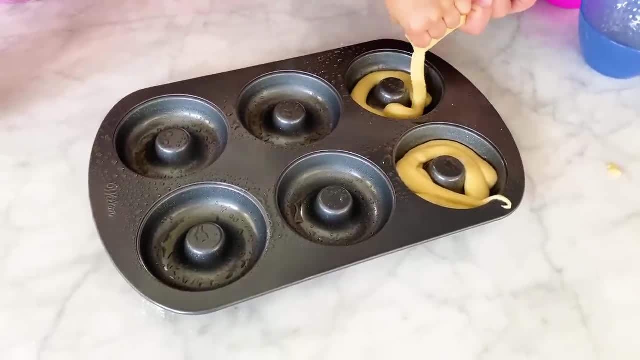 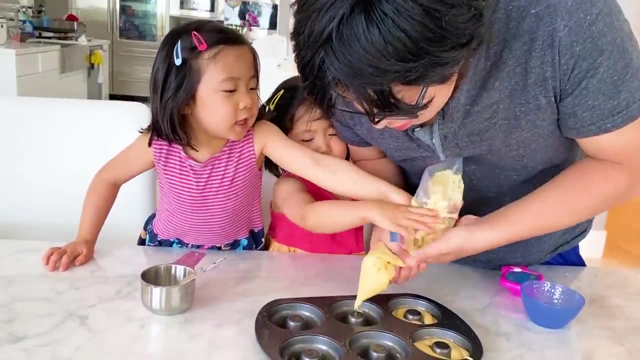 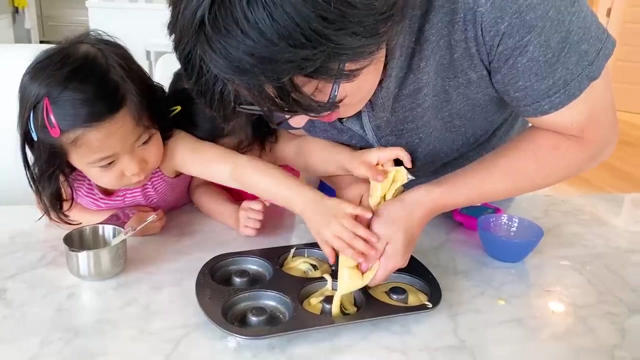 Good job, guys. Okay, Well done. Thank you for helping us a little bit. Let's see how many donuts we can make. Yeah, There you go. Okay, Daddy's strong. Yeah, Daddy's super strong, I'm strong. 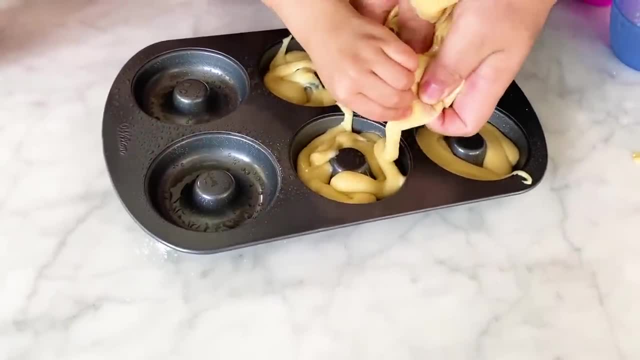 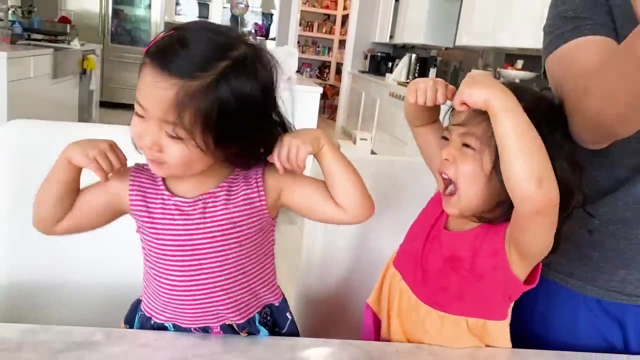 You guys are strong. Look at Emma's muscle. Yeah, Okay, here we go Put it in the oven. Thank you, Okay, All right, Emma's helping me Now. where am I going to put it? Right here, Emma. 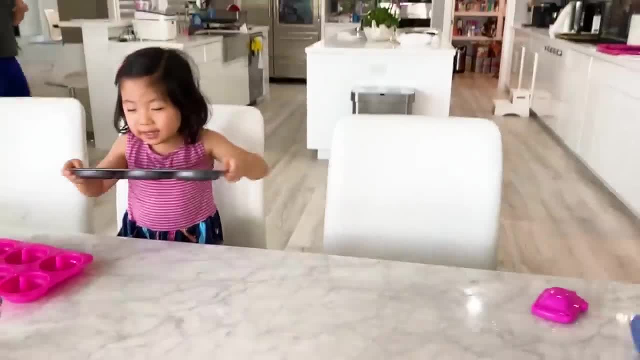 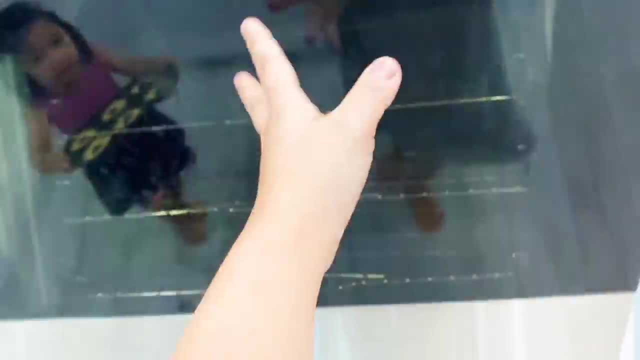 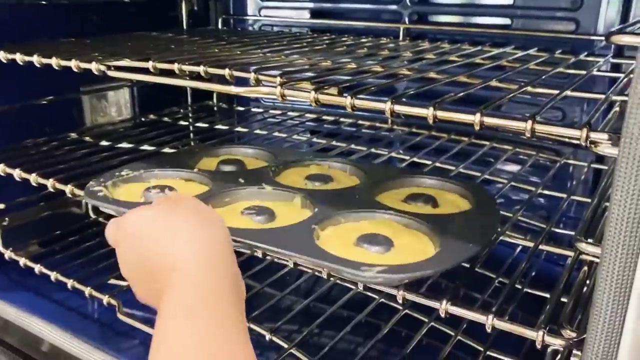 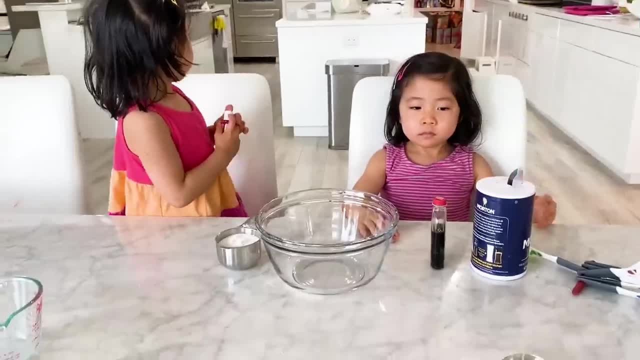 Okay, Here you go. Thank you, Emma. All right, guys. We're going to bake it for about 10 minutes. While we wait for the donut to cook, we're going to make the glaze. Okay, What glaze? 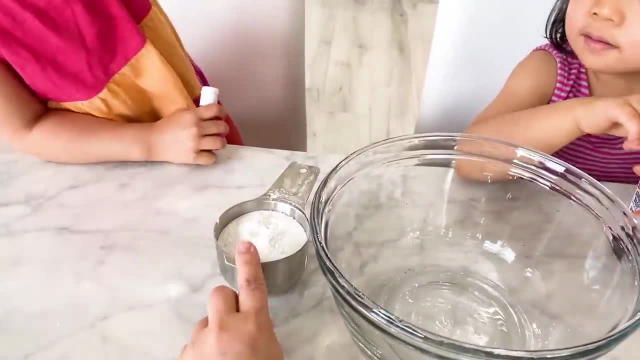 Glaze the donut. So you want sugar, donut right Sugar. Okay, So let's add in the sugar powder into here. I want a little bit. Yeah, Help each other. All of this, Yeah, all of it. 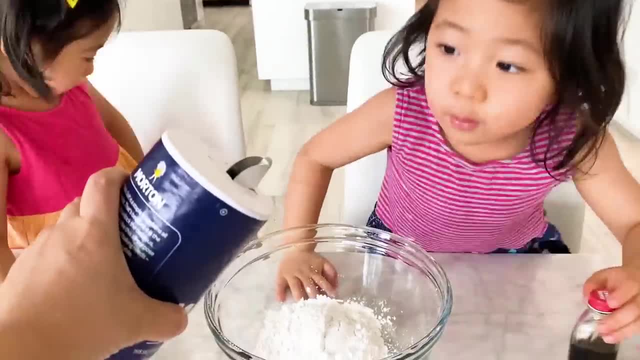 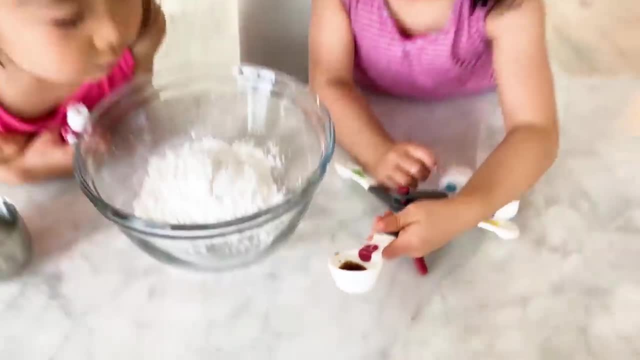 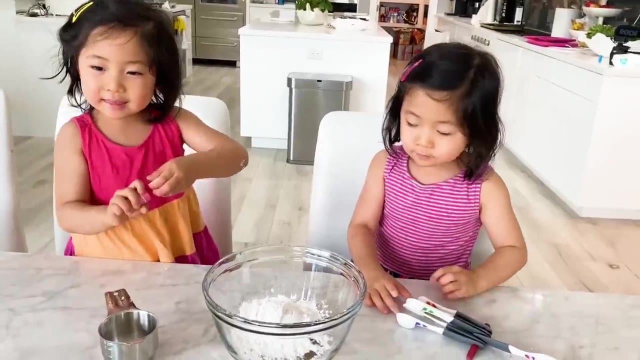 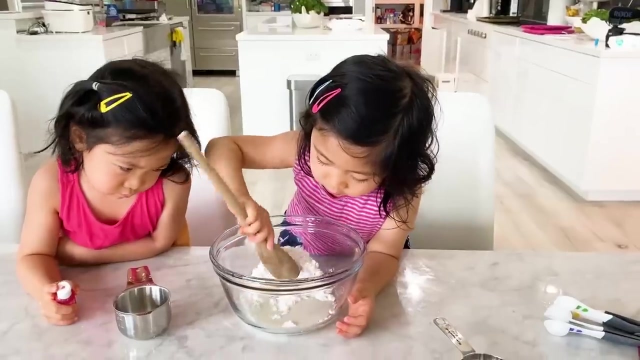 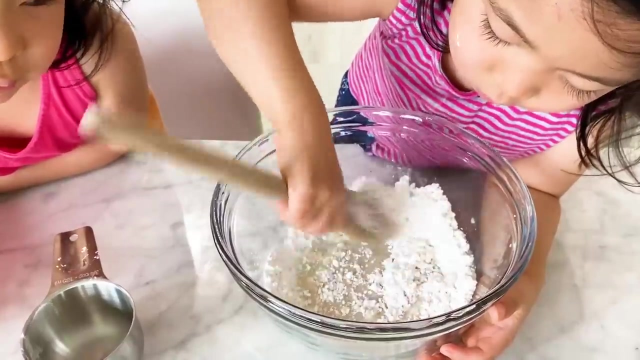 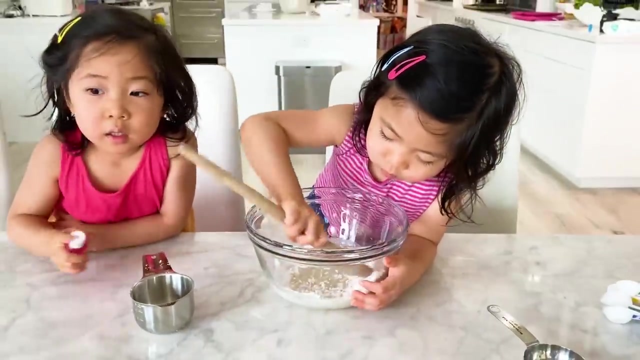 Okay, a pinch of salt, tiny bit. we're gonna add a tiny bit of vanilla extract, not a lot. there you go. let's add milk first. okay, add in the milk. okay, now we're gonna mix it together. Emma's doing great. good job, Emma. there you go, agitate, agitate, yeah, yeah, they. 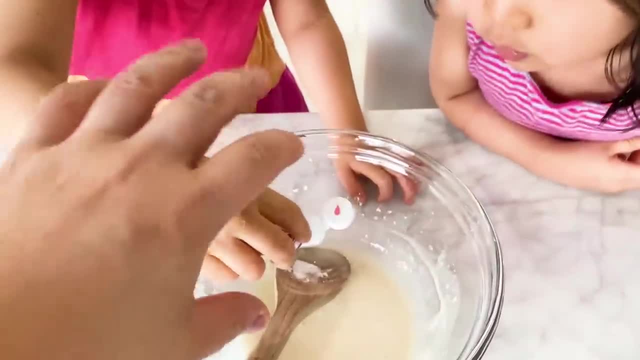 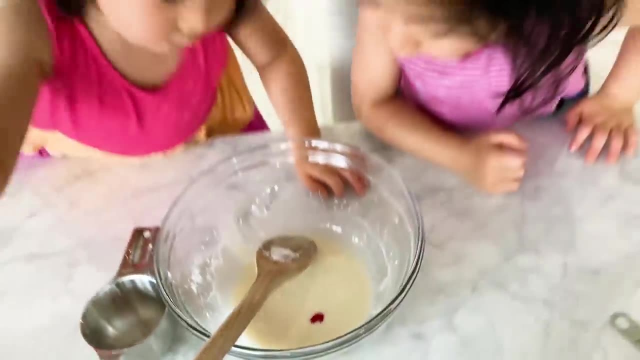 want to make a pink glaze. good job, Emma. okay, so now we're gonna add a little bit of pink. yeah, everybody help there, you go. okay, ready, you want to make a pink one? yeah, like a pink glaze. I'll hold it there. you go see how it looks. 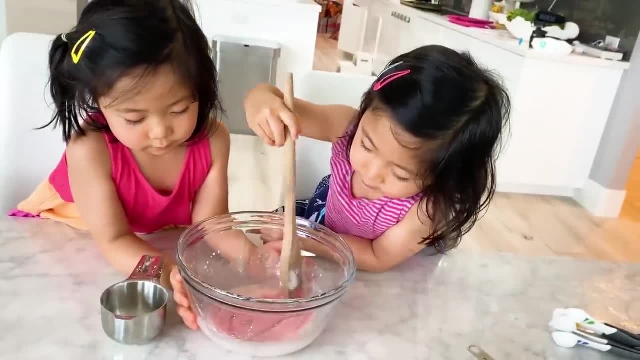 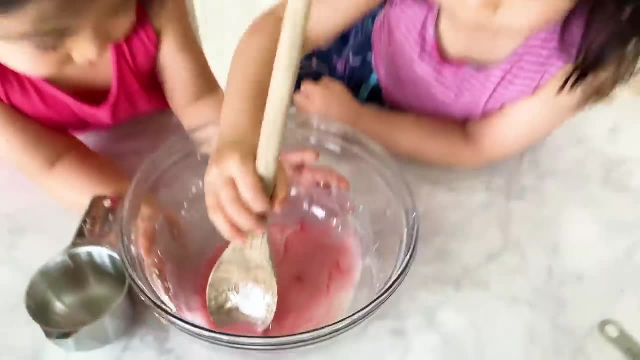 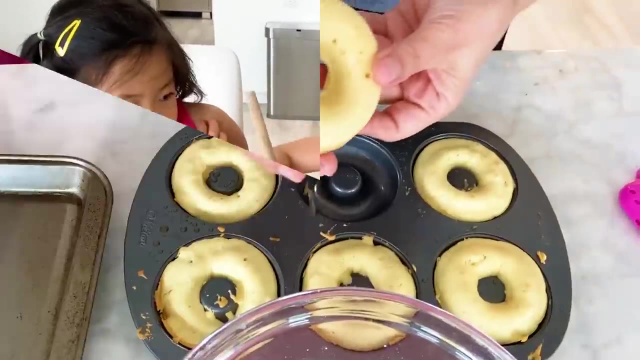 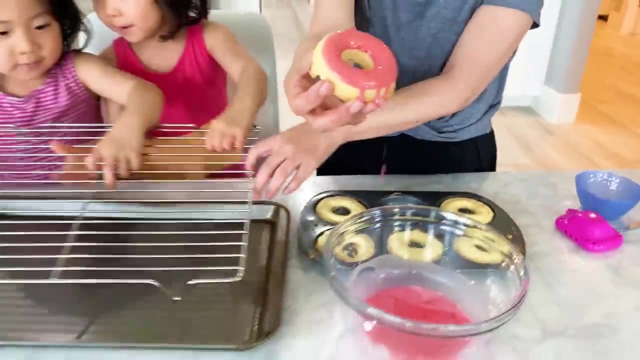 the sugar is turning pink. good teamwork, good job guys. there you go- pink, it's turning more pink. yeah, okay, guys. so now we're gonna just wait for the doughnut to be done and we'll take it out and show you guys. okay, okay, so we got it out. now we're gonna dip it in the glaze sugar, like so, and then put it to. 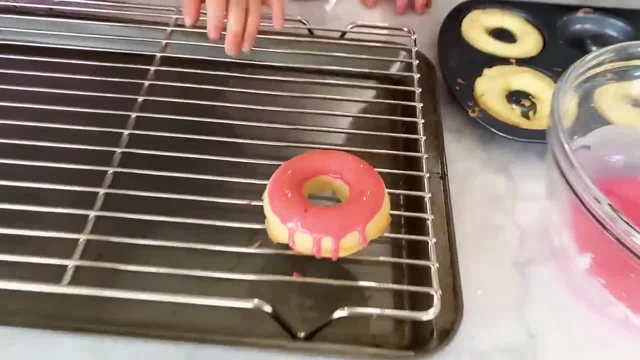 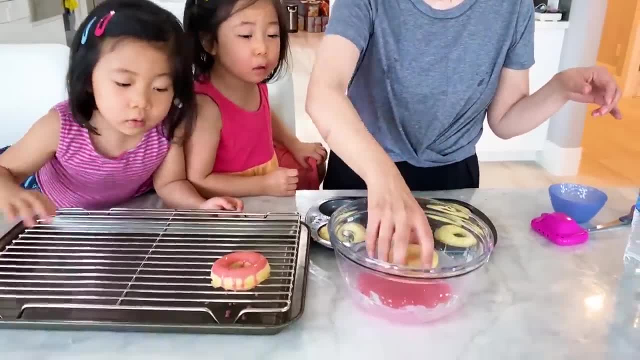 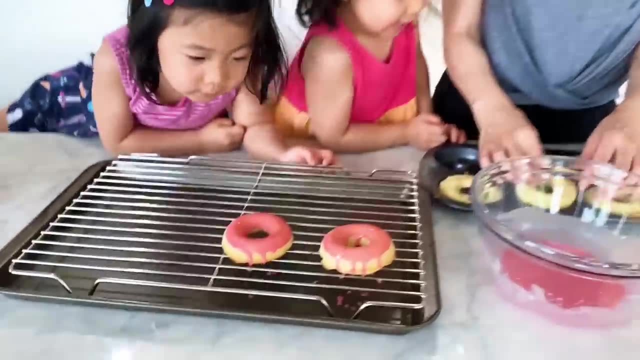 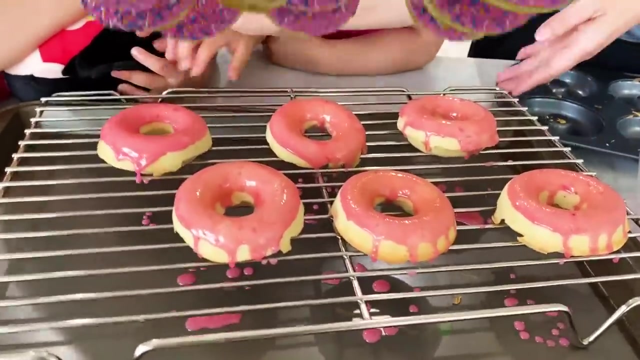 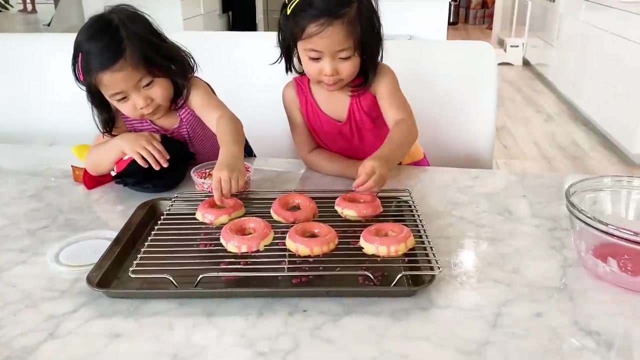 the pan, there we go, it looks good, looks good. huh, oh yeah, that's a good idea. next time we should make different color, you're right. and then you guys can do the sprinkles. okay, yeah, there's sprinkles, you guys can sprinkle it on. okay, sprinkle the doughnuts there. you. 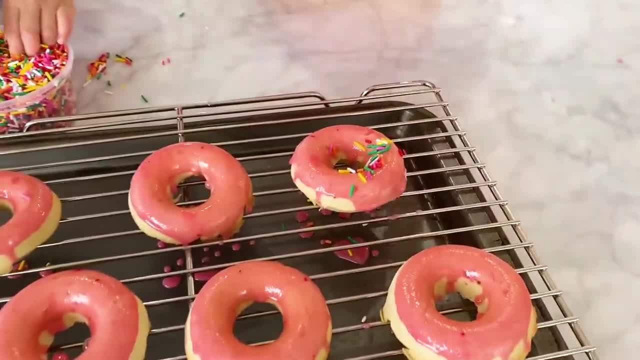 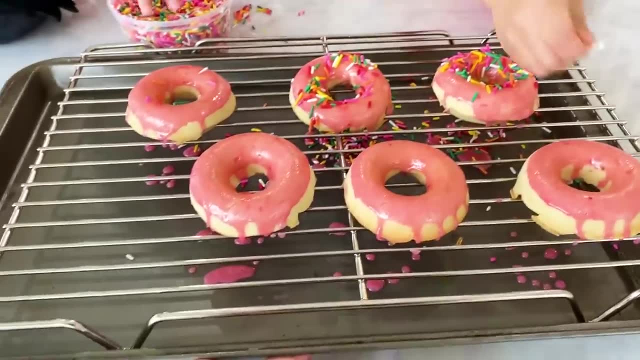 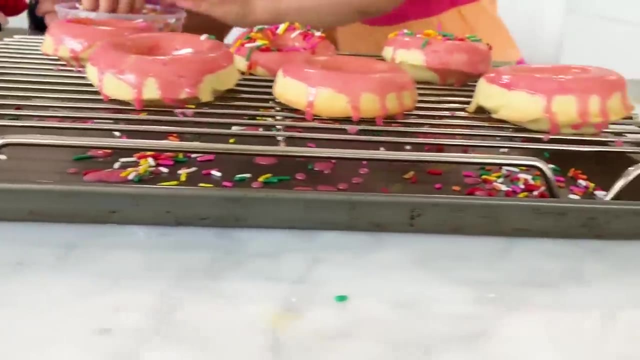 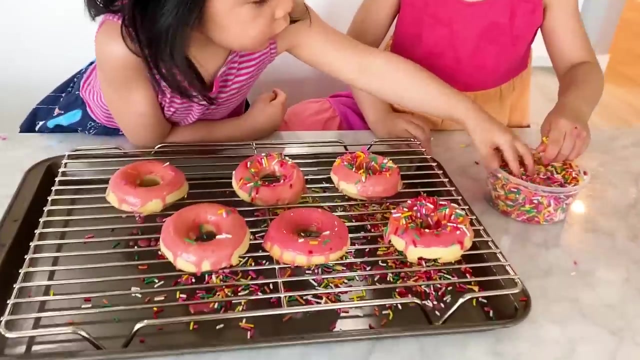 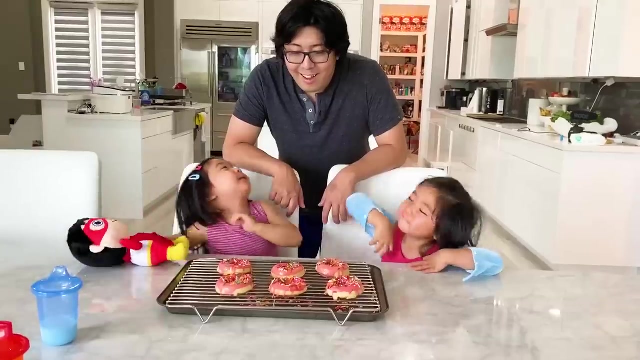 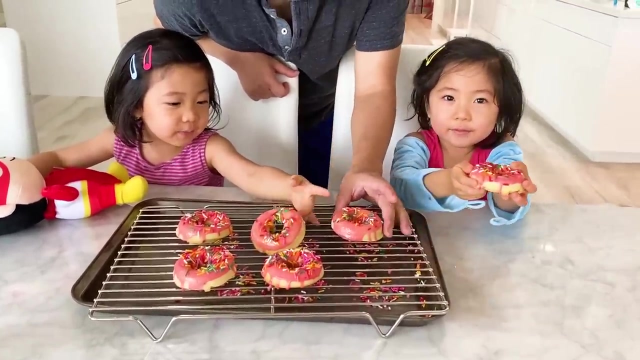 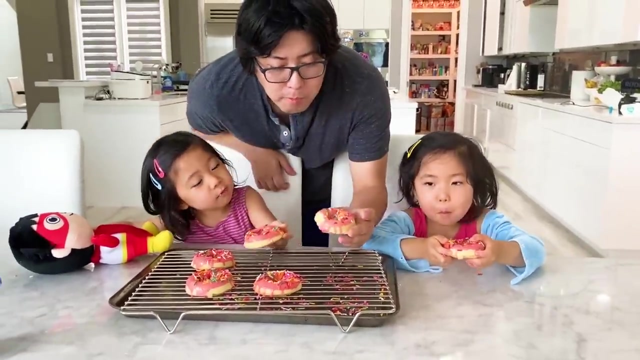 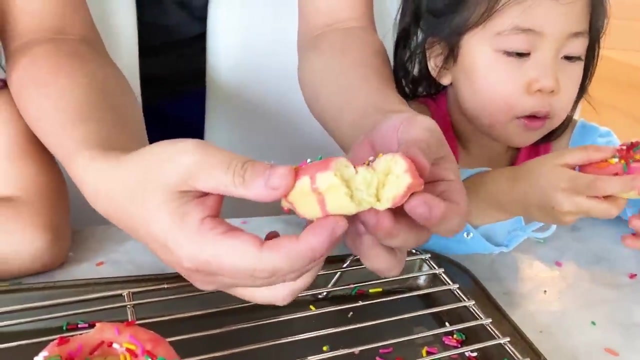 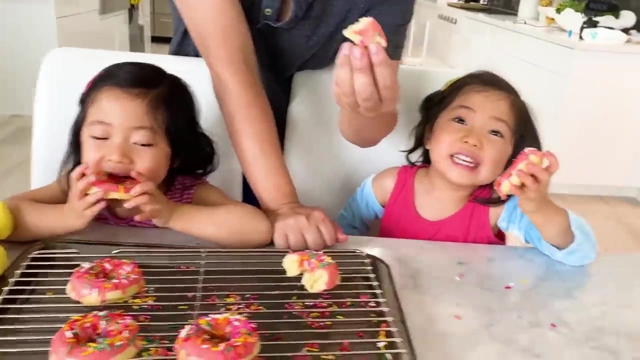